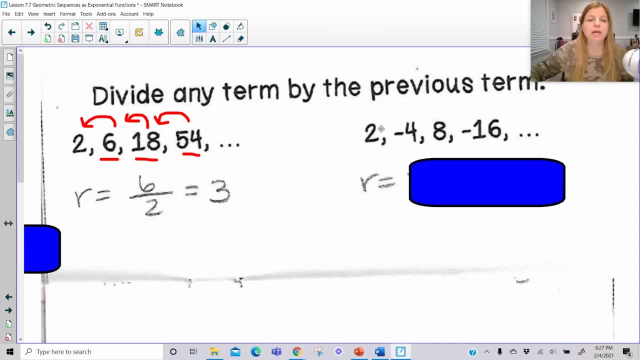 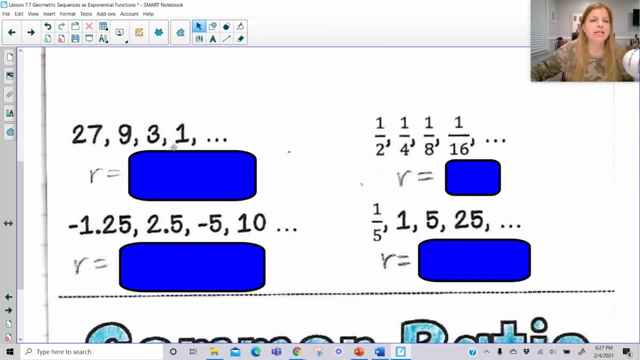 8, negative 16.. So again same idea. You may see what the multiplier is. It's multiplying by negative 2, or again, you can take any term and divide it by whatever the previous term is to get that value: 27,, 9,, 3,, 1.. If I take any term and I divide it by the previous, so 9 divided by 27,. 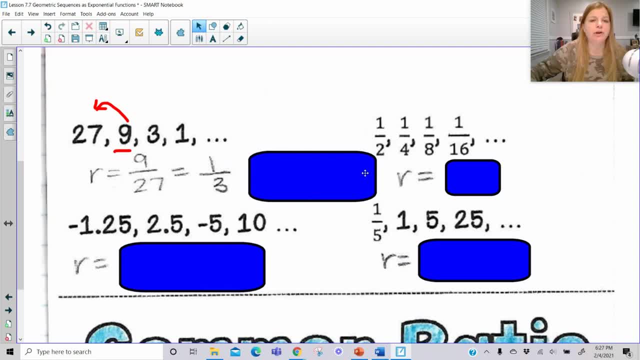 I get 9 over. 27 is not 3,, it's actually 1 third. So you may look at this sequence and be like it's not multiplying, It's actually dividing by 3.. Well, remember, dividing by 3 actually means the same thing as multiplying. 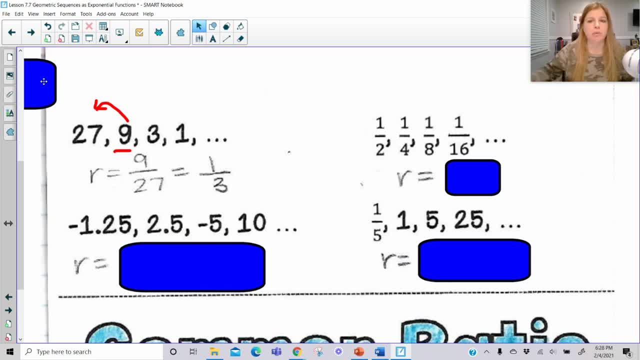 by 1 third. So we want to say the common ratio is that 1 third, 1 half, 1 fourth, 1 eighth, 1 sixteenth- I can see the numerator is staying the same. So the numerator in order to stay ones. 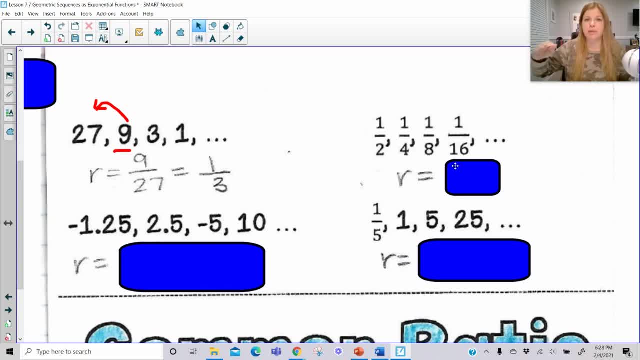 would have to be multiplied by 1.. But look, how do you go from a 2 to a 4, to an 8 to a 16? You're multiplying by 2.. This one might be a little tougher to do. Take a term and divide it. 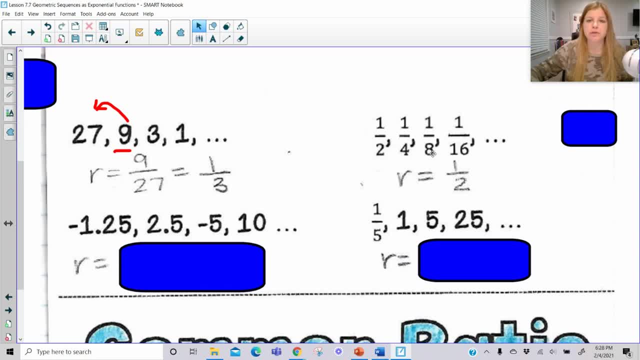 by the previous term. But as long as you can figure out what your multiplier is for your numerator and denominator, you're going to get the same thing. So you're going to have to take the denominator. You've got it Negative 1.25,, 2.5, negative 5.10.. The common ratio here is: 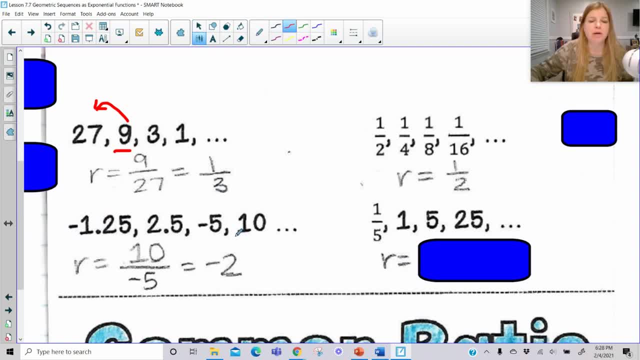 negative 2.. And again, this is an option where an example where you may want to take your integer numbers, if you can avoid decimals, in order to figure it out. So 10 divided by negative 5, is that negative 2.? And then here, 1, fifth, 1, 525.. Clearly it's multiplying by 5.. But again, 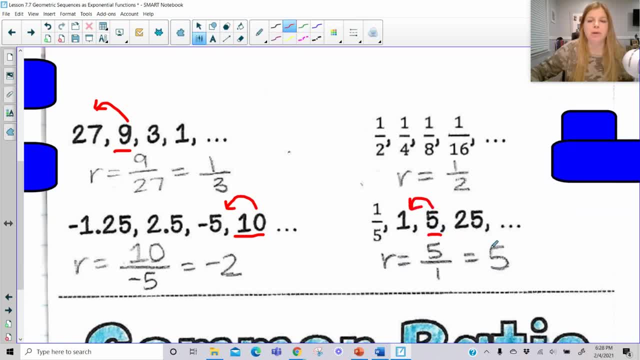 if I wanted to take any term and divide it by the previous term, I'm going to get that common ratio. So I'm going to take the denominator and divide it by the previous term, I'm going to get the common ratio. Now let's take a look at figuring out what the common ratio is. So some 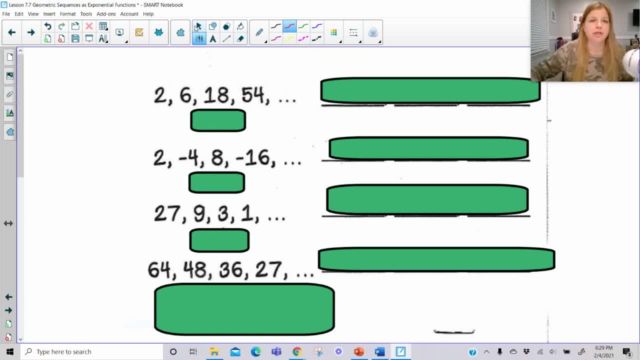 of these sequences are going to look very familiar. And then finding the next three terms. So here: 2, 6,, 18,, 54. We already saw this one. The common ratio is 3.. So that would just simply mean I would. 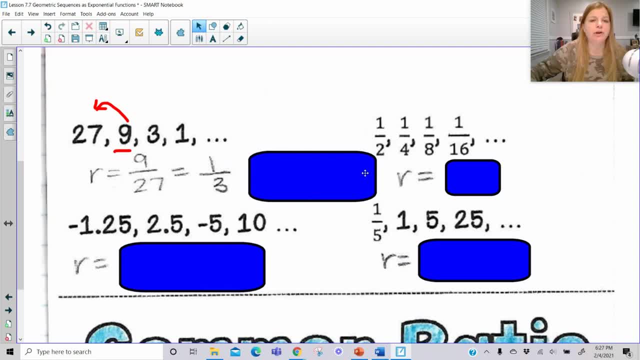 I get 9 over. 27 is not 3,, it's actually 1 third. So you may look at this sequence and be like it's not multiplying, It's actually dividing by 3.. Well, remember, dividing by 3 actually means the same thing as multiplying. 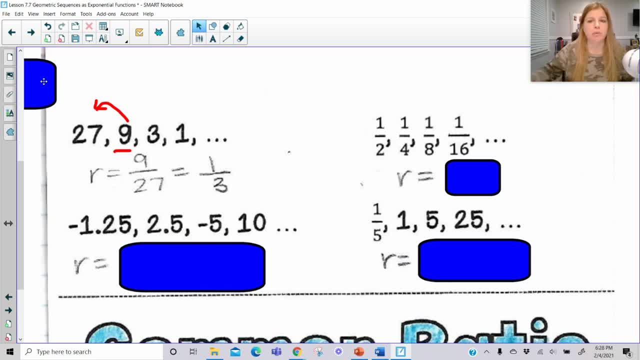 by 1 third. So we want to say the common ratio is that 1 third, 1 half, 1 fourth, 1 eighth, 1 sixteenth- I can see the numerator is staying the same. So the numerator in order to stay ones. 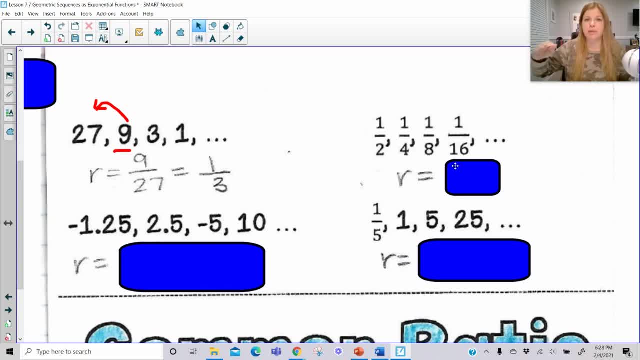 would have to be multiplied by 1.. But look, how do you go from a 2 to a 4, to an 8 to a 16? You're multiplying by 2.. This one might be a little tougher to do. Take a term and divide it. 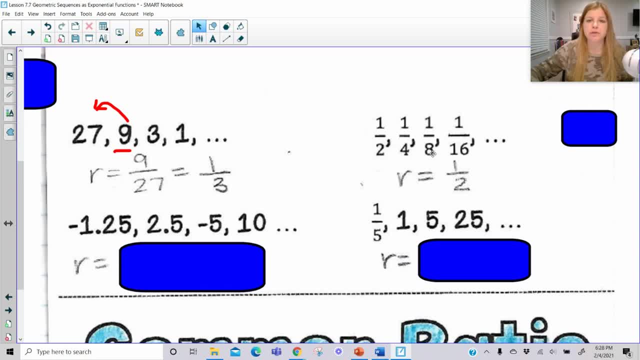 by the previous term. But as long as you can figure out what your multiplier is for your numerator and denominator, you're going to get the same thing. So you're going to have to take the denominator. You've got it Negative 1.25,, 2.5, negative 5.10.. The common ratio here is: 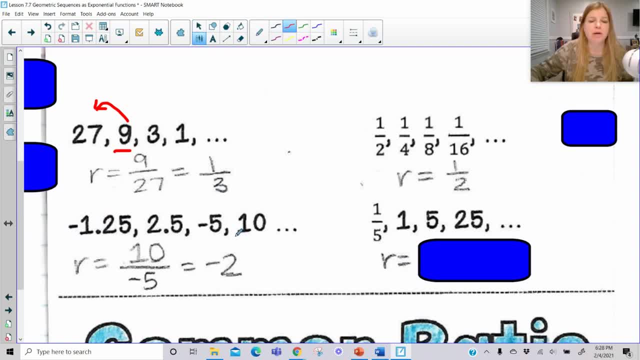 negative 2.. And again, this is an option where an example where you may want to take your integer numbers, if you can avoid decimals, in order to figure it out. So 10 divided by negative 5, is that negative 2.? And then here, 1, fifth, 1, 525.. Clearly it's multiplying by 5.. But again, 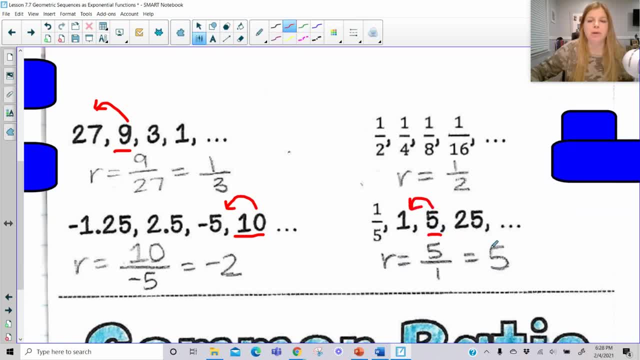 if I wanted to take any term and divide it by the previous term, I'm going to get that common ratio. So I'm going to take the denominator and divide it by the previous term, I'm going to get that common ratio. Now let's take a look at figuring out what the common ratio is. So some 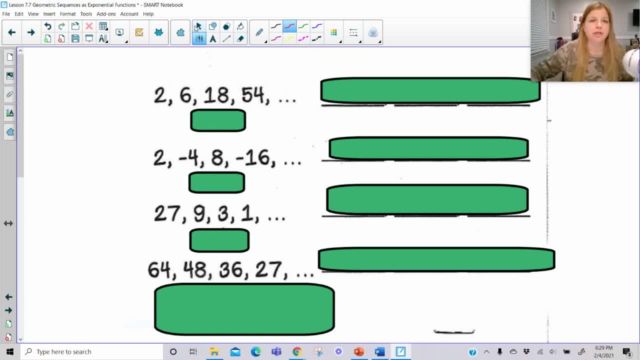 of these sequences are going to look very familiar. And then finding the next three terms. So here: 2, 6,, 18,, 54. We already saw this one. The common ratio is 3.. So that would just simply mean I would. 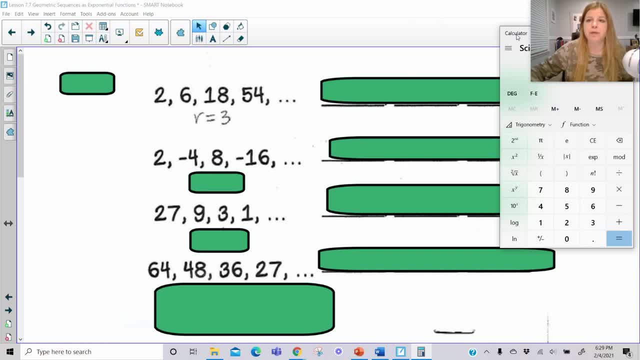 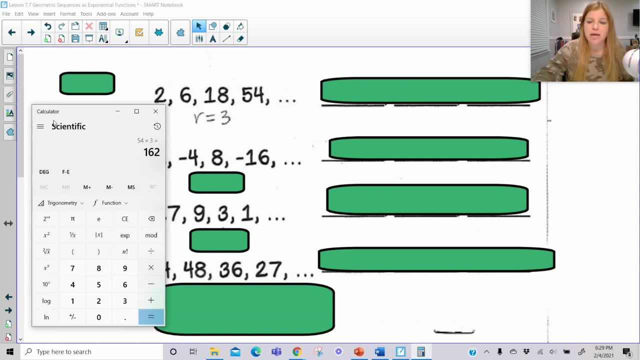 to extend this pattern, take 54.. I'll just move my calculator over And just simply multiply it by 3.. And I get 162.. So I would write 162 down, And then I'm going to multiply that by 3. And I get 486.. So 162, 486.. And if I multiply 486 by 3, I'm going to get 1458.. 2, negative 4,. 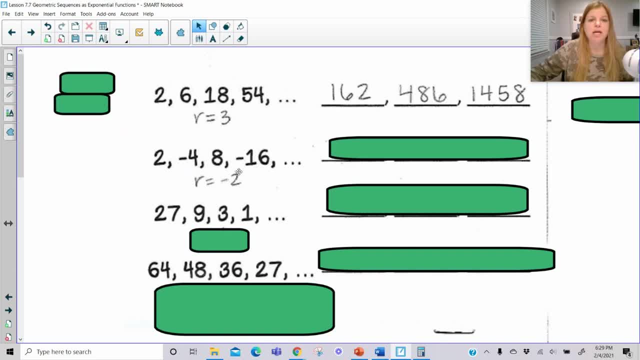 8, negative 16. My common ratio is negative 2.. If I continue to multiply by negative 2, what you're going to see in a pattern like this: anytime the common ratio is negative, you're going to be alternating between positives and negatives Because- think about it- A positive 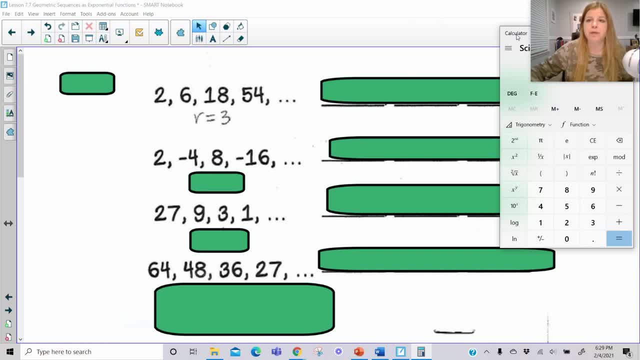 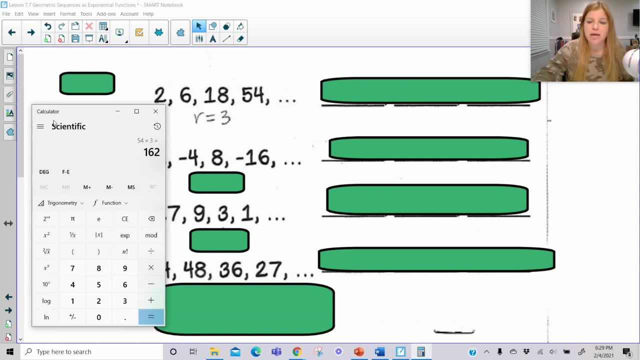 to extend this pattern, take 54.. I'll just move my calculator over And just simply multiply it by 3.. And I get 162.. So I would write 162 down, And then I'm going to multiply that by 3. And I get 486.. So 162, 486.. And if I multiply 486 by 3, I'm going to get 1458.. 2, negative 4,. 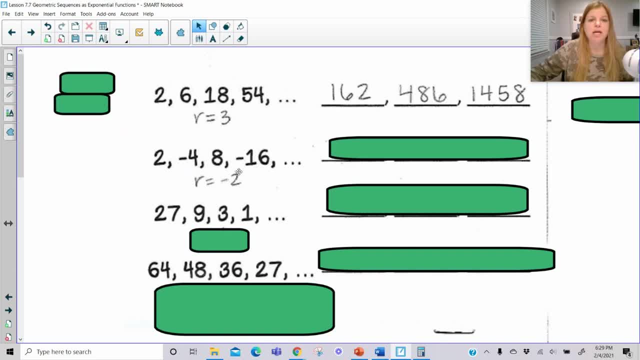 8, negative 16. My common ratio is negative 2.. If I continue to multiply by negative 2, what you're going to see in a pattern like this: anytime the common ratio is negative, you're going to be alternating between positives and negatives Because- think about it- A positive 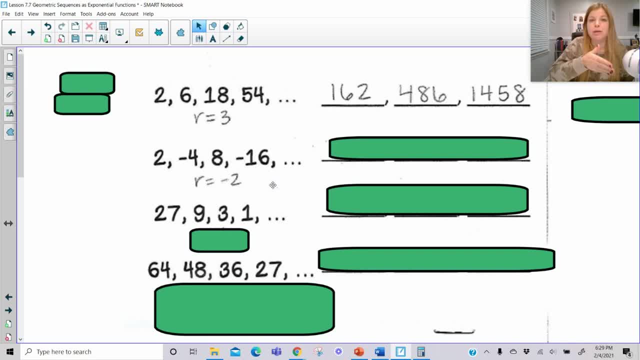 times a negative is negative And then when you take that negative value and multiply it by the negative, you're going to get 1458.. So if I continue to multiply by negative 2, I'm going to get 1458.. So if I continue to multiply by negative 2, I'm going to get 1458.. So if I continue to, 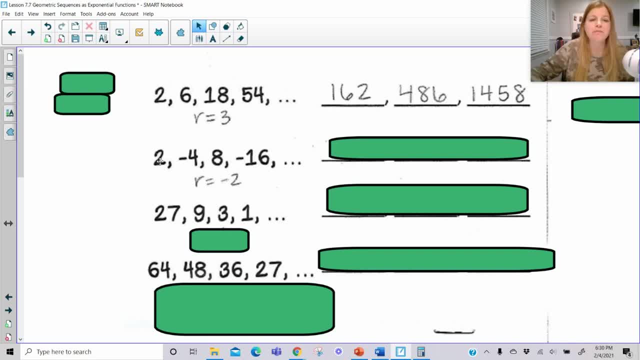 common ratio, it's going to go back to positive. So if I have positive 2, negative 4, positive 8, negative 16,, the next term would be positive 32, then negative 64, and then positive 128. 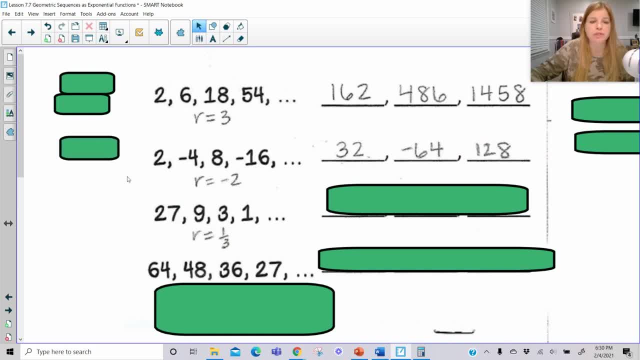 27,, 9,, 3,, 1, we can know the common ratio is one-third. We saw that before. So if I keep multiplying by one-third or dividing by 3, my next term would be one-third Now one-third divided by 3, or one-third multiplied by one-third. 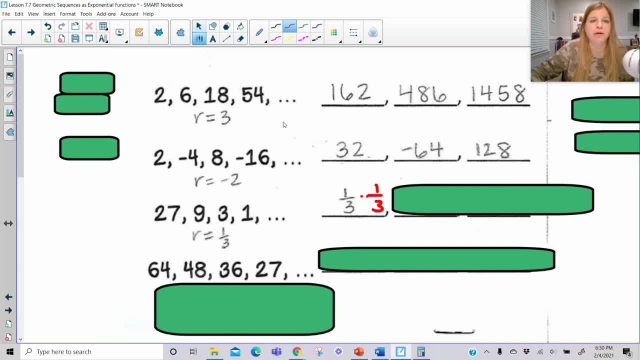 remember that's what we're really doing. We're multiplying by one-third, So one-third times one-third is one-ninth, And then one-ninth times one-third would be- I'm sure you're saying it, I hope you're saying it- give us 1 over 27.. Okay, 64, 48,, 36, 27.. This one might not be as obvious. 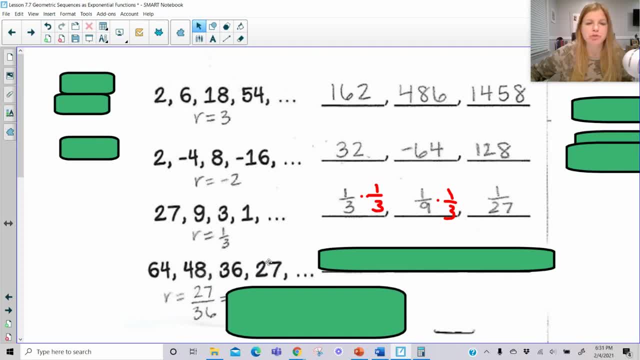 but if I go ahead and I take any term and divide it by the previous, so 27 over 36, I end up getting a fraction of three-fourths, or I can use the decimal equivalent. Either one is honestly fine to call it the common ratio. So three-fourths or 0.75.. 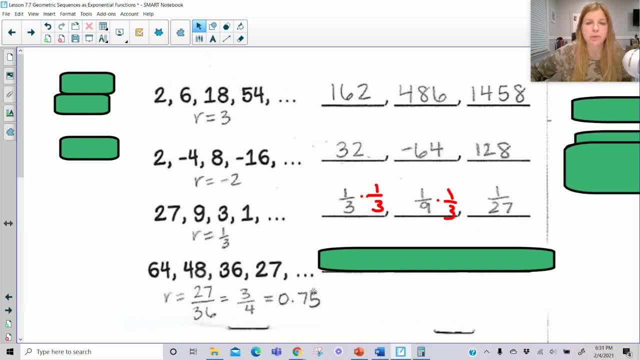 And if I continue that and I multiply 27 times 0.75, I'm going to get 20.25.. And 20.25 times 0.75 is 15.1875.. And then this value multiplied by 0.75,. 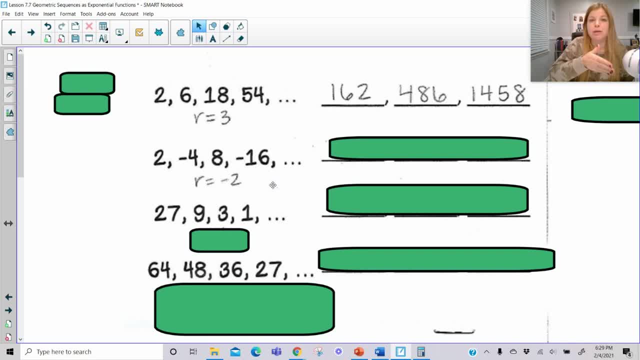 times a negative is negative And then when you take that negative value and multiply it by the negative, you're going to get 1458.. So if I continue to multiply by negative 2, I'm going to get 1458.. So if I continue to multiply by negative 2, I'm going to get 1458.. So if I continue to, 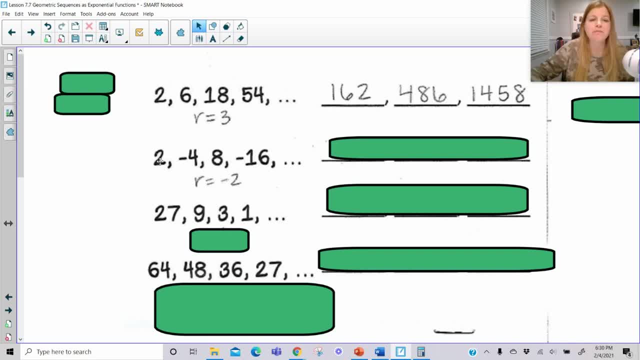 common ratio, it's going to go back to positive. So if I have positive 2, negative 4, positive 8, negative 16,, the next term would be positive 32, then negative 64, and then positive 128. 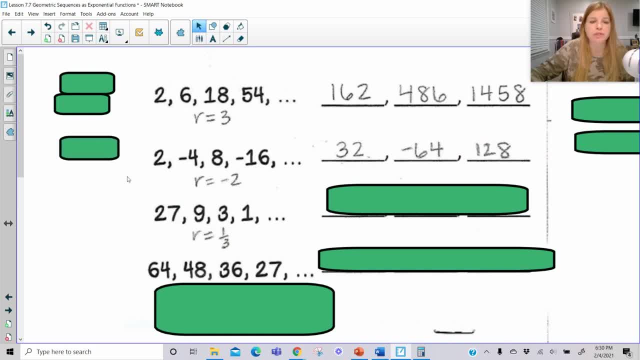 27,, 9,, 3,, 1, we can know the common ratio is one-third. We saw that before. So if I keep multiplying by one-third or dividing by 3, my next term would be one-third Now one-third divided by 3, or one-third multiplied by one-third. 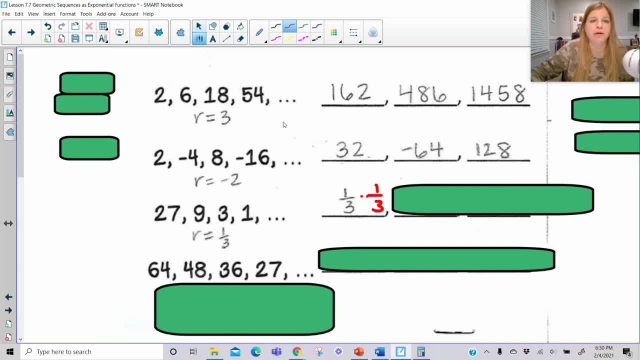 remember that's what we're really doing. We're multiplying by one-third, So one-third times one-third is one-ninth, And then one-ninth times one-third would be- I'm sure you're saying it, I hope you're saying it- give us 1 over 27.. Okay, 64, 48,, 36, 27.. This one might not be as obvious. 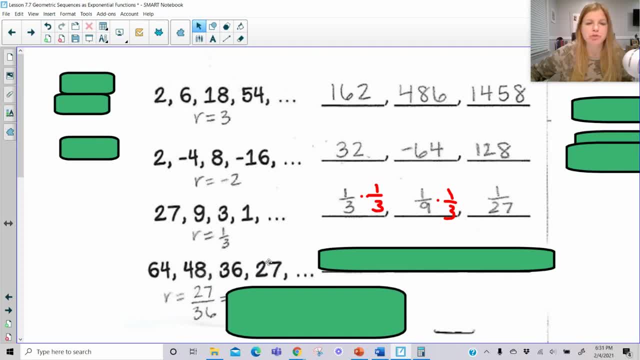 but if I go ahead and I take any term and divide it by the previous, so 27 over 36, I end up getting a fraction of three-fourths, or I can use the decimal equivalent. Either one is honestly fine to call it the common ratio. So three-fourths or 0.75.. 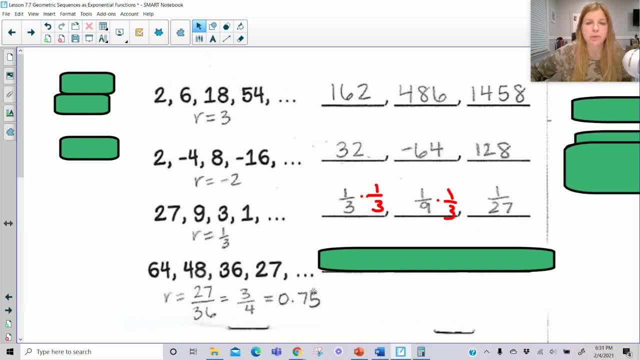 And if I continue that and I multiply 27 times 0.75, I'm going to get 20.25.. And 20.25 times 0.75 is 15.1875.. And then this value multiplied by 0.75,. 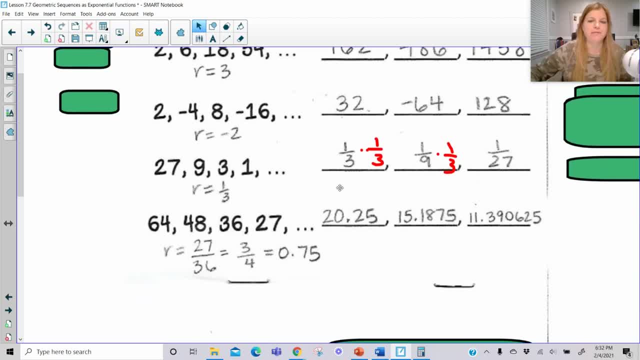 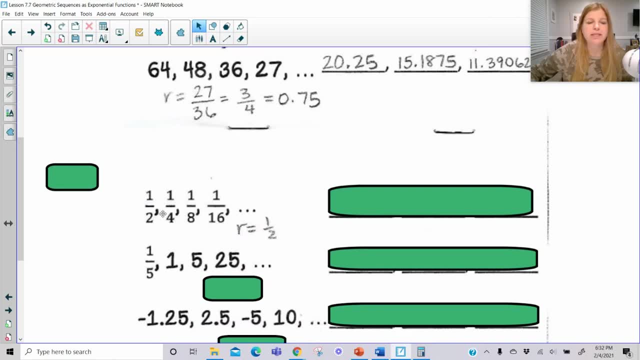 you can see, is this: 11.390625.. Okay, one-half, one-fourth, one-eighth, one-sixteenth. we know the common ratio Here is one-half. So if I continue, remember, I'm really just keeping ones at the top. 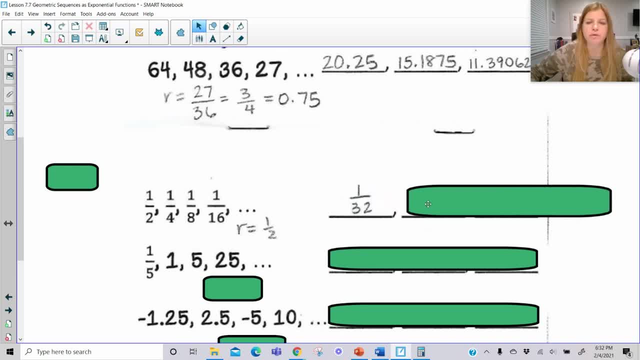 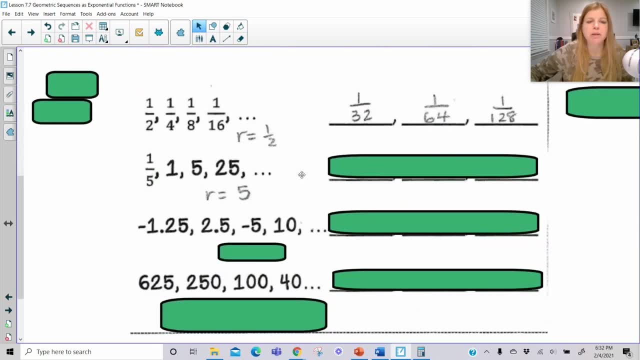 but I'm multiplying my denominators by two, So the next one would be 1 over 32,, 1 over 64,, 1 over 28.. The common ratio here is five. We saw this in a previous problem. So if I continue to multiply five, I'm going to get 125, 625, and 3125. 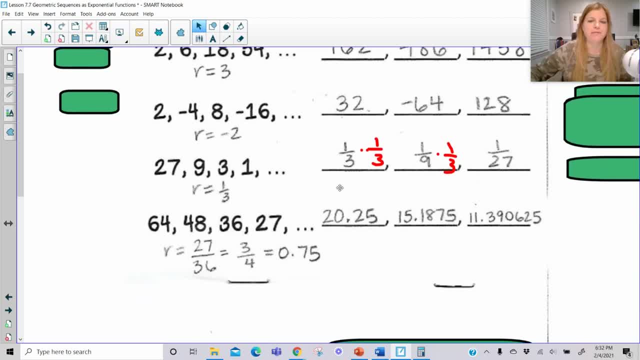 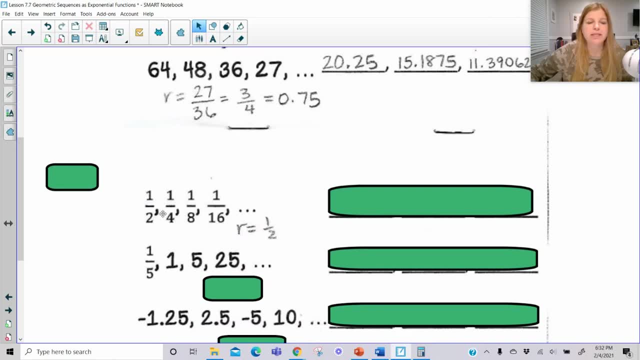 you can see, is this: 11.390625.. Okay, one-half, one-fourth, one-eighth, one-sixteenth. we know the common ratio Here is one-half. So if I continue, remember, I'm really just keeping ones at the top. 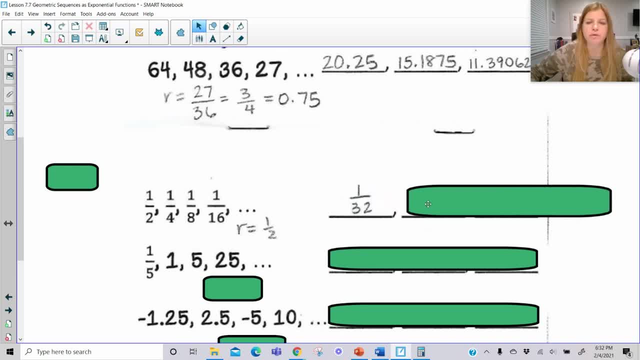 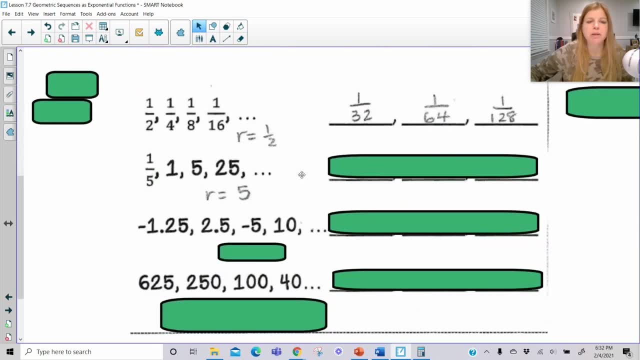 but I'm multiplying my denominators by two, So the next one would be 1 over 32,, 1 over 64,, 1 over 28.. The common ratio here is five. We saw this in a previous problem. So if I continue to multiply five, I'm going to get 125, 625, and 3125. 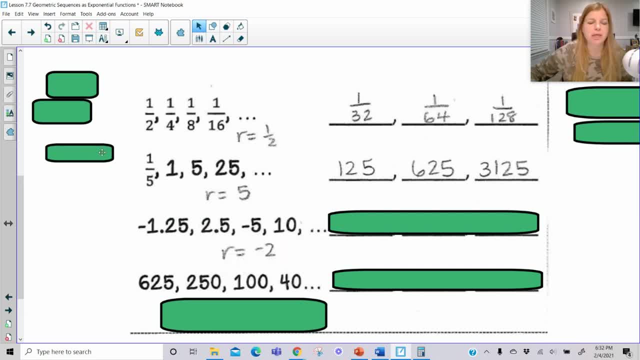 This is another one. we already found the common ratio for. It's multiplying by negative two. So if we continue to multiply by negative two, multiply by negative, multiply by negative two. Remember, anytime the common ratio is negative, you're going to have these alternating positives and negatives. 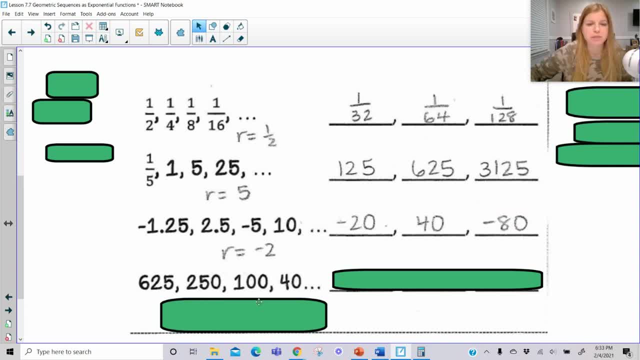 This last one. here is another example where we may not figure out the common ratio just by looking at it. So we definitely need to set up a fraction where we take any number and term and divide it by the previous term. So if I do 40 divided by 100, I'm going to get two-fifths or 0.4.. 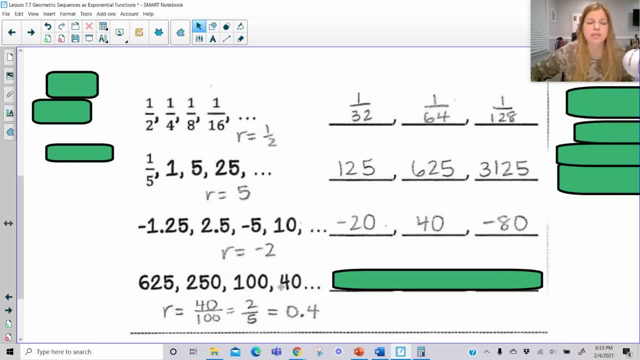 Then I can take either the two-fifths or the 0.4 and continue the sequence and do 40 times that 0.4 is 16.. So I'm going to take either the two-fifths or the 0.4 and continue the sequence. 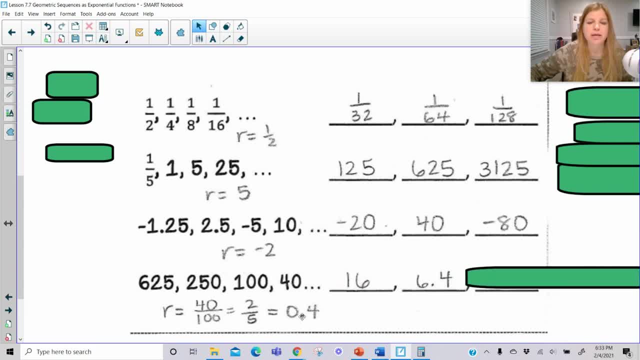 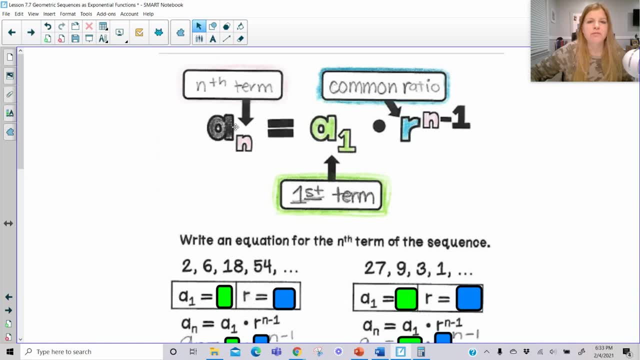 16 times 0.4 is 6.4, and 6.4 times 0.4 is 2.56.. Now for this really kind of funky looking formula: a sub n- remember subscripts. we say a sub n is. 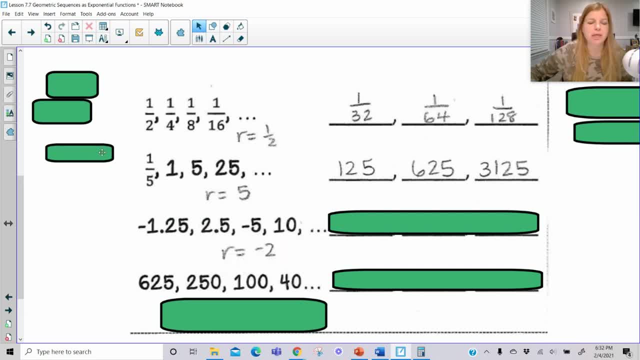 This is another one. we already found the common ratio for. It's multiplying by negative two. So if we continue to multiply by negative two, multiply by negative, multiply by negative two. Remember, anytime the common ratio is negative, you're going to have these alternating positives and negatives. 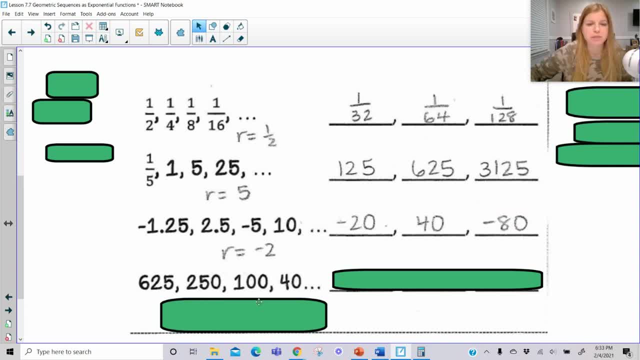 This last one. here is another example where we may not figure out the common ratio just by looking at it. So we definitely need to set up a fraction where we take any number and term and divide it by the previous term. So if I do 40 divided by 100, I'm going to get two-fifths or 0.4.. 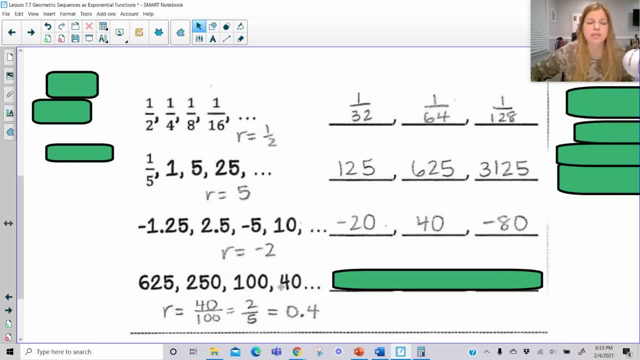 Then I can take either the two-fifths or the 0.4 and continue the sequence and do 40 times that 0.4 is 16.. So I'm going to take either the two-fifths or the 0.4 and continue the sequence. 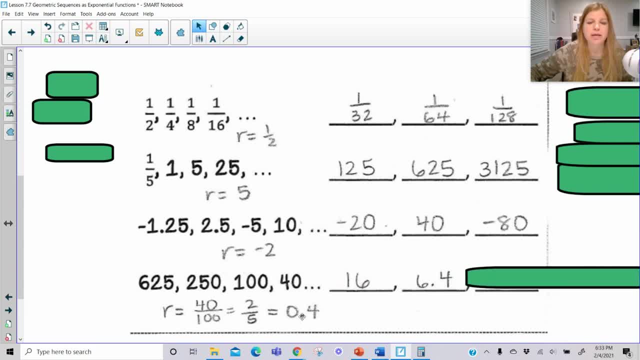 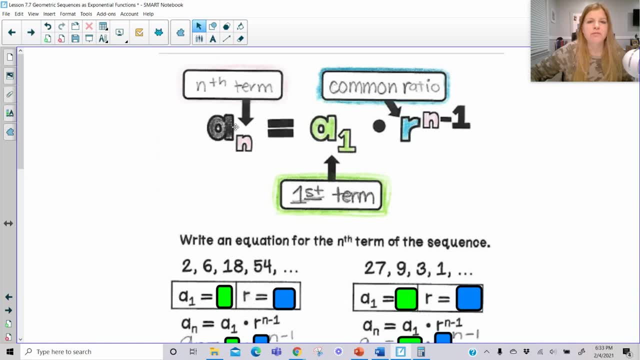 16 times 0.4 is 6.4, and 6.4 times 0.4 is 2.56.. Now for this really kind of funky looking formula: a sub n- remember subscripts. we say a sub n is. 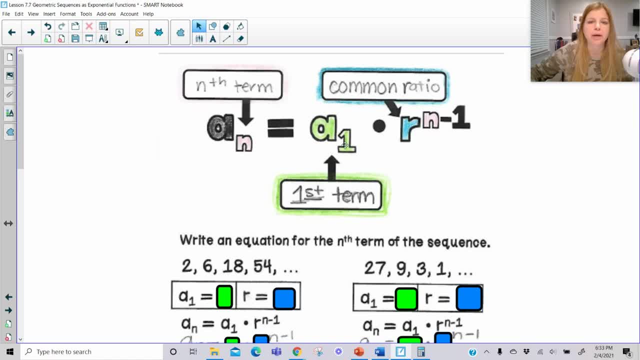 equal to a sub 1.. We've seen a sub 1 before, We should remember. a sub 1 means the first term in the sequence is then multiplied by whatever. the common ratio r is to the n minus 1, power. And remember n just means what term in the sequence we want to solve for. 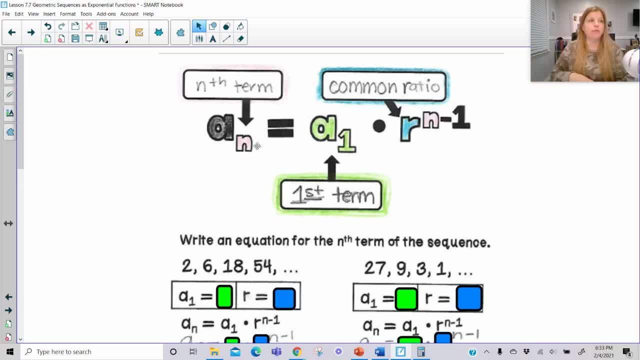 And using formulas like this are super helpful. If I gave you a sequence that was, you know, 5, and then 10,, 20,, 40,, I'm multiplying by 2.. And I ask you for, like the 36th term in the 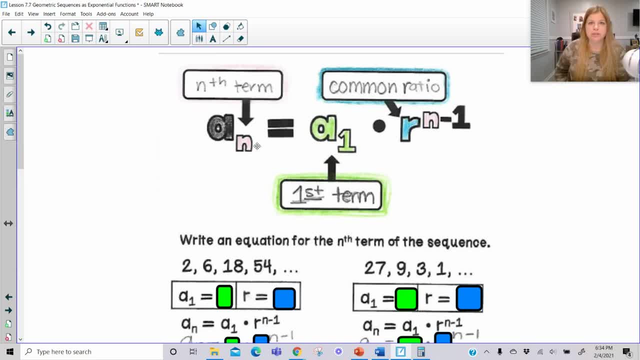 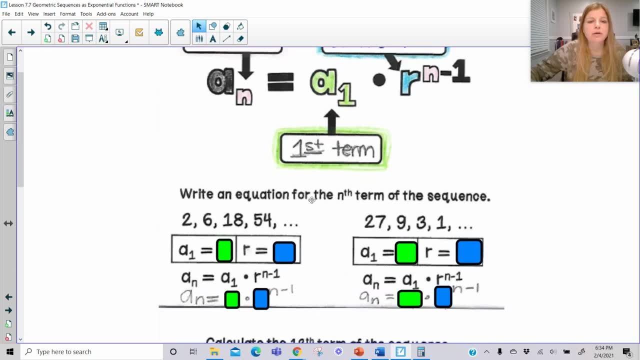 sequence. Well, you're not going to want to multiply out that sequence 32 more times. If you just plug the values into this formula, you're going to get your answer pretty quickly. So here it says: write an equation for the nth term. 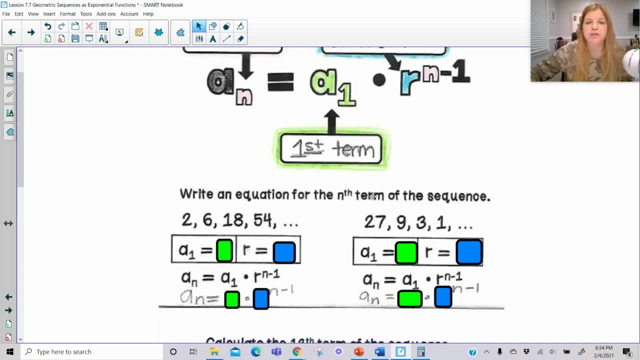 And remember any time you have a problem that says write an equation for the nth term, that means you get to leave n in the formula. So where you see n in these two spots in the formula, that stays. So we're really just replacing the a sub 1 and replacing the common ratio r. 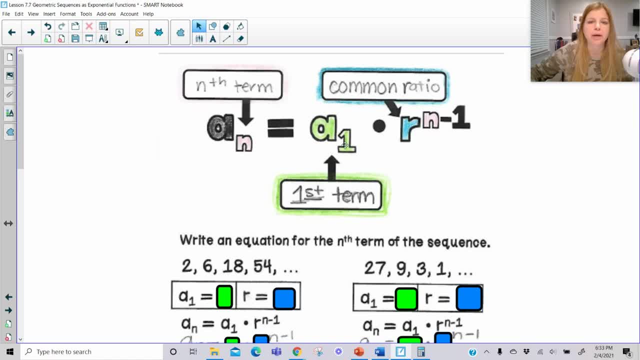 equal to a sub 1.. We've seen a sub 1 before, We should remember. a sub 1 means the first term in the sequence is then multiplied by whatever. the common ratio r is to the n minus 1, power. And remember n just means what term in the sequence we want to solve for. 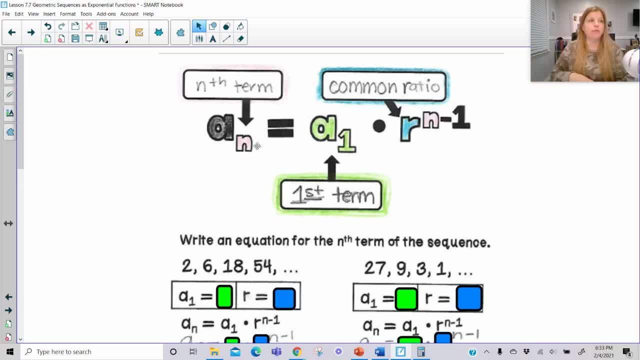 And using formulas like this are super helpful. If I gave you a sequence that was, you know, 5, and then 10,, 20,, 40,, I'm multiplying by 2.. And I ask you for, like the 36th term in the 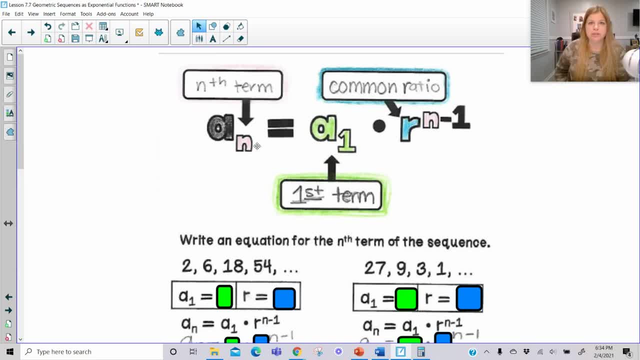 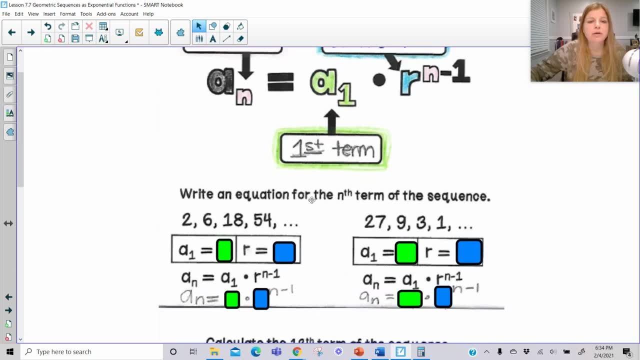 sequence. Well, you're not going to want to multiply out that sequence 32 more times. If you just plug the values into this formula, you're going to get your answer pretty quickly. So here it says: write an equation for the nth term. 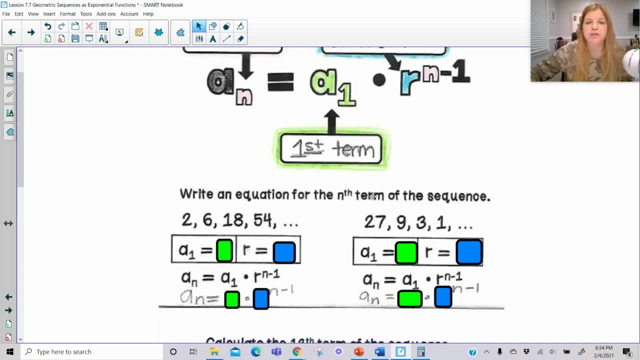 And remember any time you have a problem that says write an equation for the nth term, that means you get to leave n in the formula. So where you see n in these two spots in the formula, that stays. So we're really just replacing the a sub 1 and replacing the common ratio r. 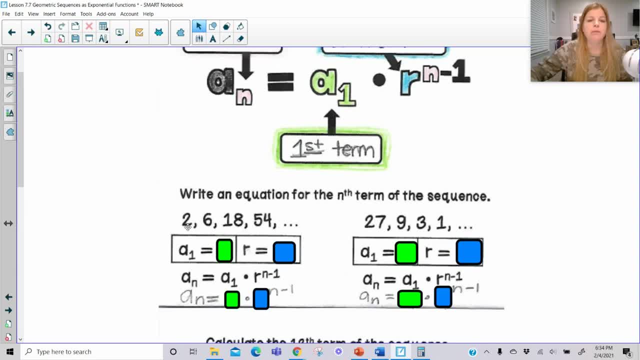 So in this sequence- and again both of these sequences we've already seen before- my a sub 1 is 2.. Remember, a sub 1 means the first term in the sequence. My common ratio is 3.. So my formula is just simply: a sub n equals. 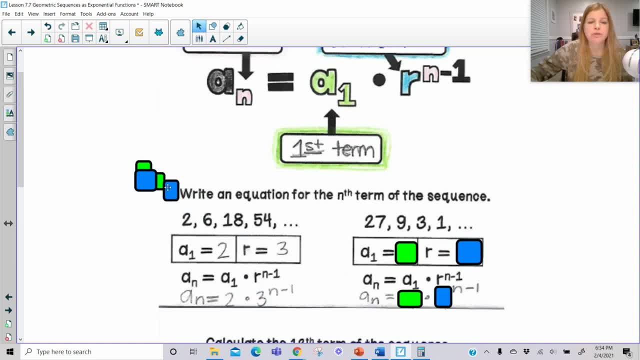 2 times 3 to the n minus 1 power. And now listen to me, do not multiply the 2 and 3 together and make it 6. That's going to be wrong Because, remember, exponents come before multiplying. 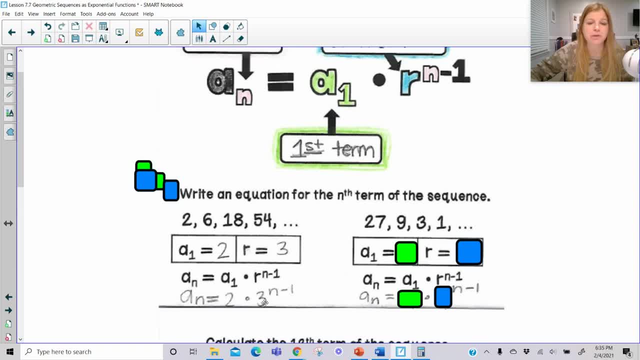 So you'd actually have to calculate 3 to the n minus 1 power first and then take that result and multiply it by 2.. So, trust me, you just leave the formula the way that looks. Next one: 27,, 9,, 3,, 1.. So my a sub 1 here is 27.. My common ratio: we see we're multiplying. 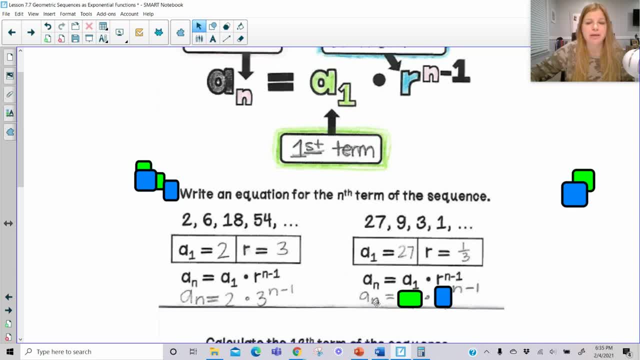 by 1 third. So my formula is simply: a sub n equals 27 times 1 third to the n minus 1 power. And again, don't make 27 times 1 third be 9.. It's going to be wrong, Trust me. that is the. 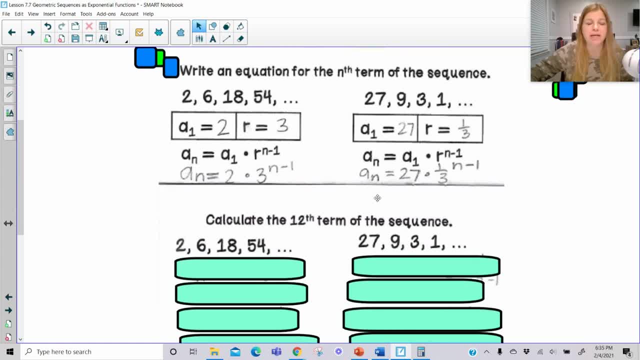 final answer. Now here's the whole point of writing out the sequence. like I mentioned before, Now that we've written our formulas, if I then said to you, find the 12th term in the sequence, Well, 12th term, you might be like, oh, that's not that many terms. I could go out. 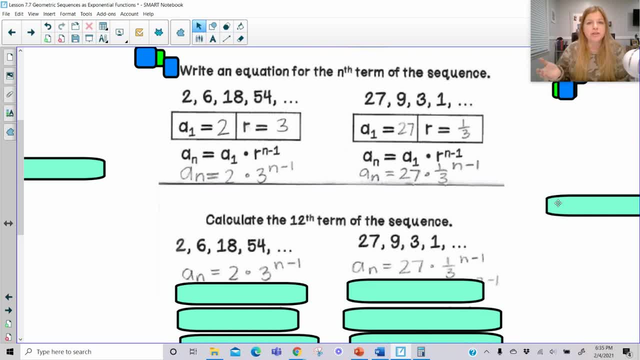 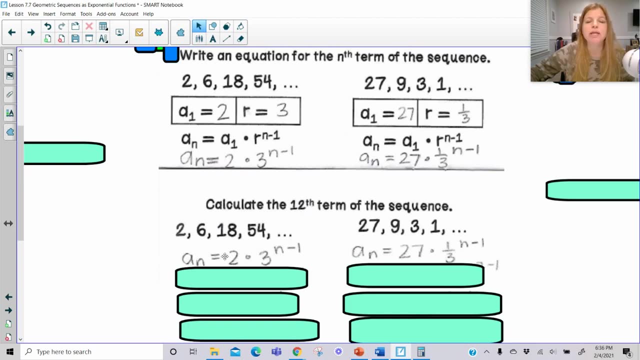 12 terms. What if I said the 45th term of the sequence That we're probably not going to want to do mentally or just by hand, or keep typing things into a calculator? So whatever term you want to solve for 12, remember that gets substituted in for n And there's two places. 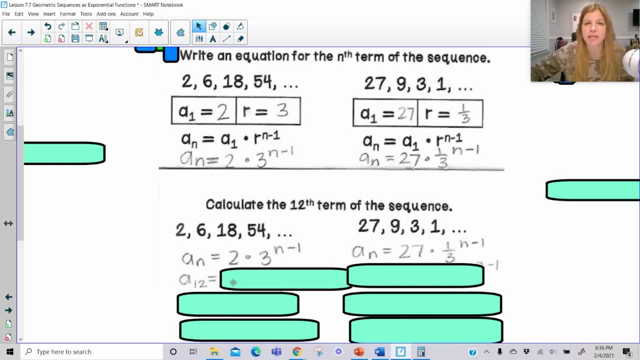 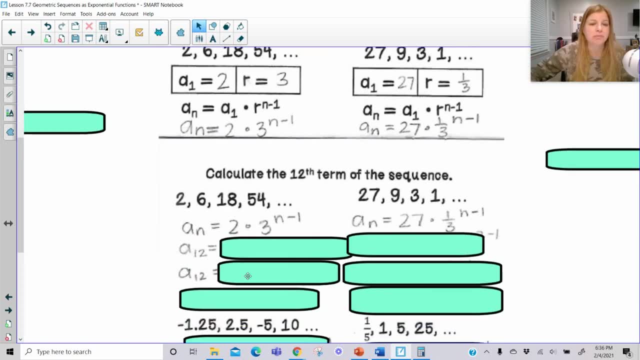 where n are. So a sub 12, remember, that's just notation, It's not a times 12.. It doesn't become 12 a. You're literally going to see it. just say a sub 12 equals a sub 12 equals. 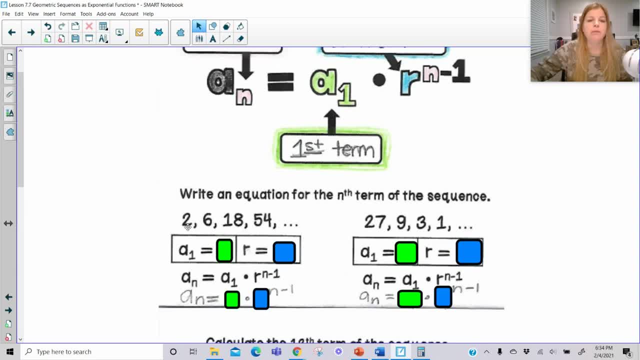 So in this sequence- and again both of these sequences we've already seen before- my a sub 1 is 2.. Remember, a sub 1 means the first term in the sequence. My common ratio is 3.. So my formula is just simply: a sub n equals. 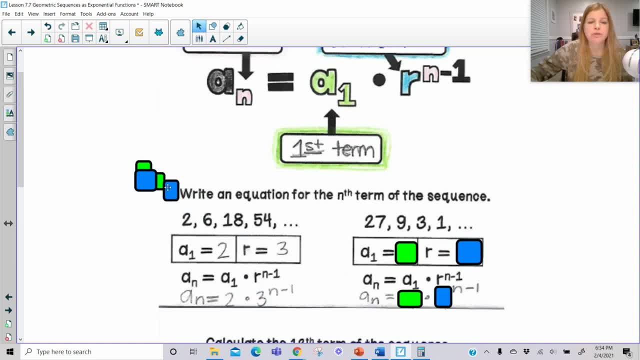 2 times 3 to the n minus 1 power. And now listen to me, do not multiply the 2 and 3 together and make it 6. That's going to be wrong Because, remember, exponents come before multiplying. 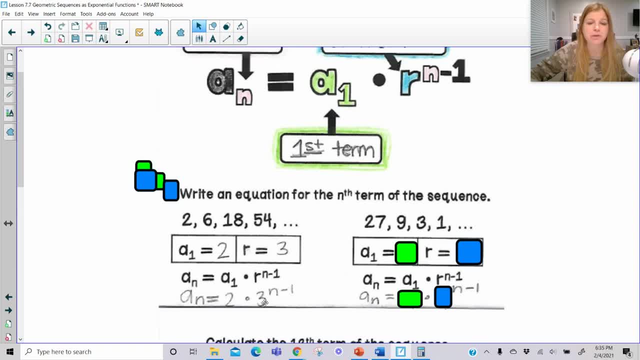 So you'd actually have to calculate 3 to the n minus 1 power first and then take that result and multiply it by 2.. So, trust me, you just leave the formula the way that looks. Next one: 27,, 9,, 3,, 1.. So my a sub 1 here is 27.. My common ratio: we see we're multiplying. 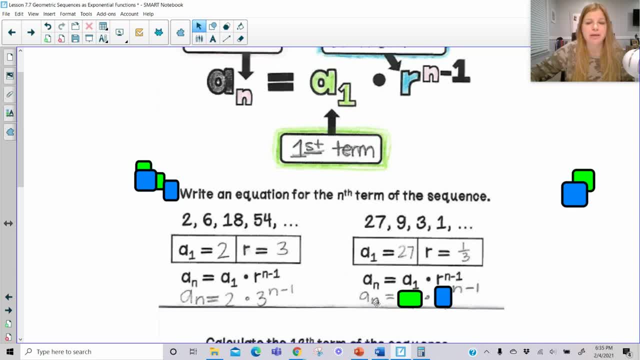 by 1 third. So my formula is simply: a sub n equals 27 times 1 third to the n minus 1 power. And again, don't make 27 times 1 third be 9.. It's going to be wrong, Trust me. that is the. 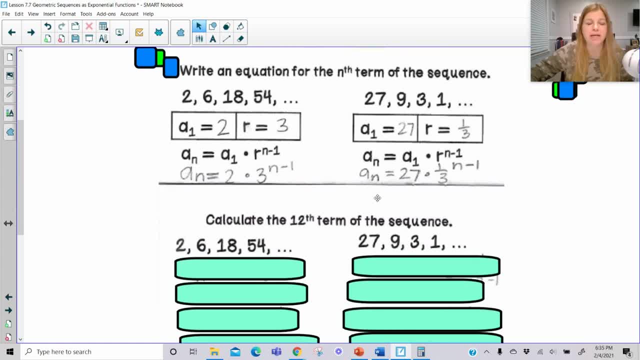 final answer. Now here's the whole point of writing out the sequence. like I mentioned before, Now that we've written our formulas, if I then said to you, find the 12th term in the sequence, Well, 12th term, you might be like, oh, that's not that many terms. I could go out. 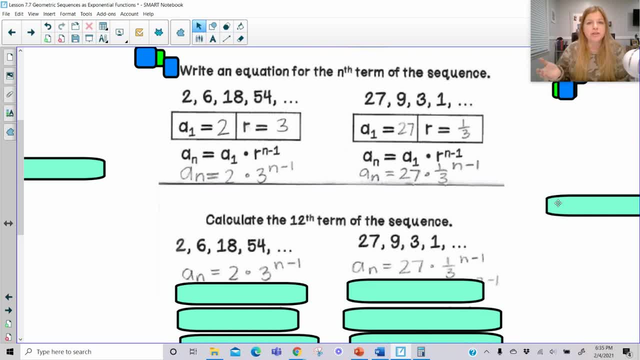 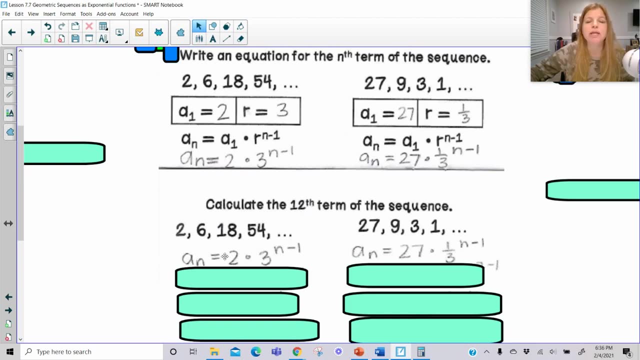 12 terms. What if I said the 45th term of the sequence That we're probably not going to want to do mentally or just by hand, or keep typing things into a calculator? So whatever term you want to solve for 12, remember that gets substituted in for n And there's two places. 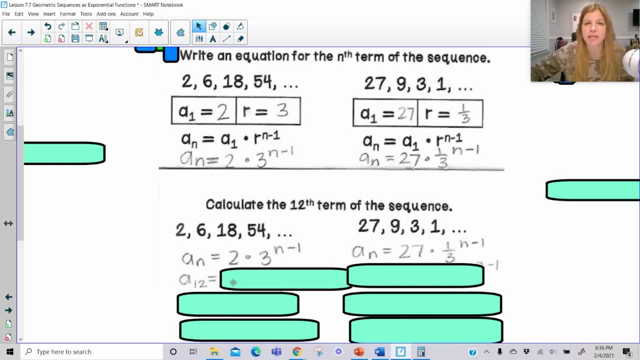 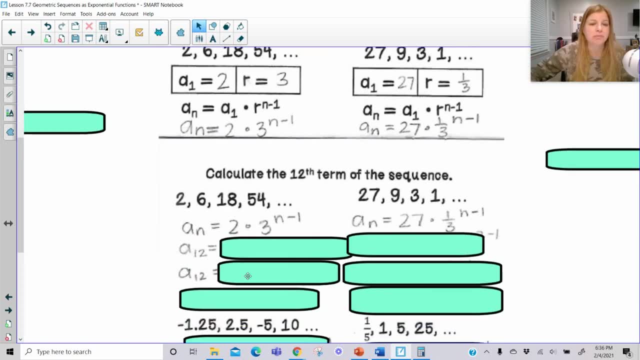 where n are. So a sub 12, remember, that's just notation, It's not a times 12.. It doesn't become 12 a. You're literally going to see it. just say a sub 12 equals a sub 12 equals. 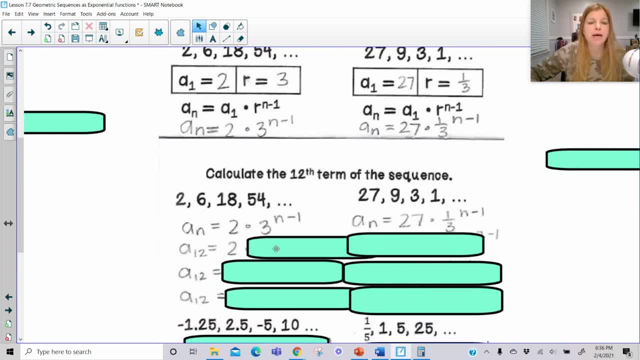 Because we're solving for the 12th term, 2 times 3 to the 12 minus 1 power. Well, 12 minus 1 is clearly 11.. And so now, if I was grabbing my calculator, I would do 3 to the 11th power. 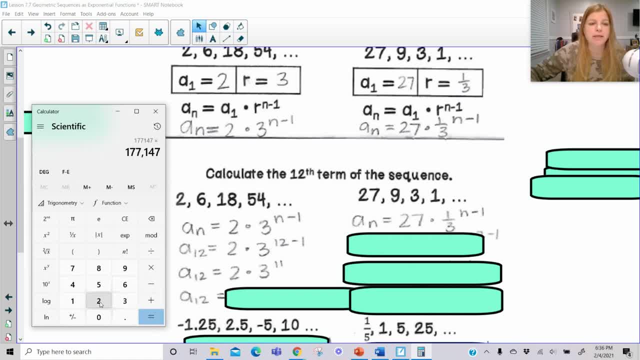 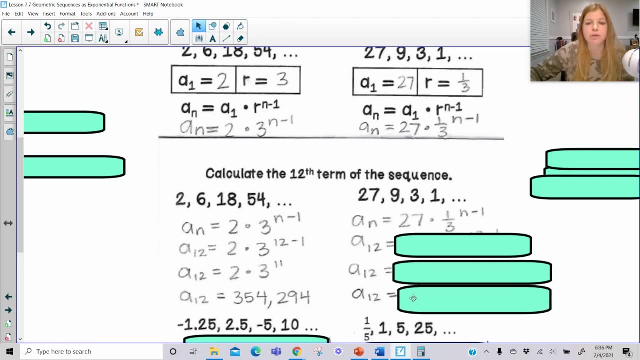 That's what comes first, And then multiply that answer by 2.. And that's my result: 354,294.. Same thing here. So if I wanted to find the 12th term, notice, it's going to say a sub 12 equals a sub 12 equals. I'm plugging in a 12 for n. I had an. 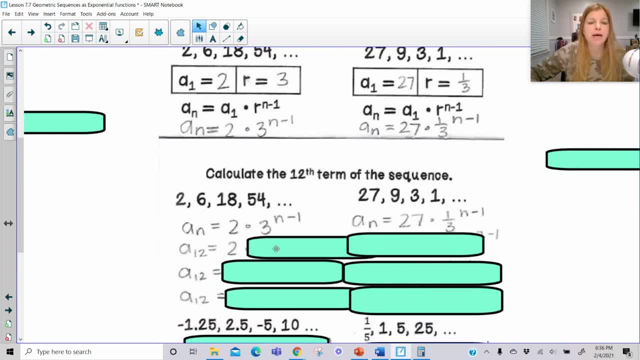 Because we're solving for the 12th term, 2 times 3 to the 12 minus 1 power. Well, 12 minus 1 is clearly 11.. And so now, if I was grabbing my calculator, I would do 3 to the 11th power. 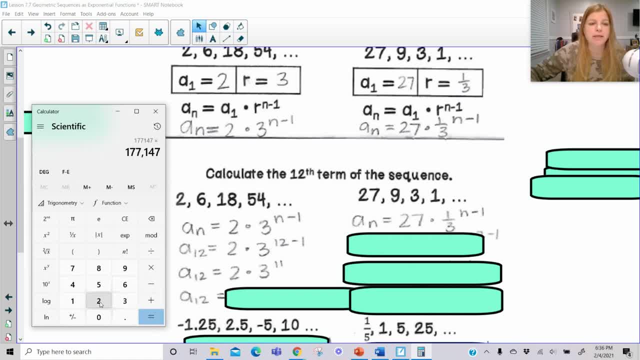 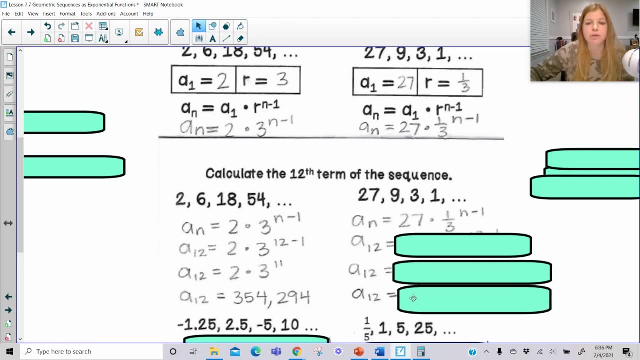 That's what comes first, And then multiply that answer by 2.. And that's my result: 354,294.. Same thing here. So if I wanted to find the 12th term, notice, it's going to say a sub 12 equals a sub 12 equals. I'm plugging in a 12 for n. I had an. 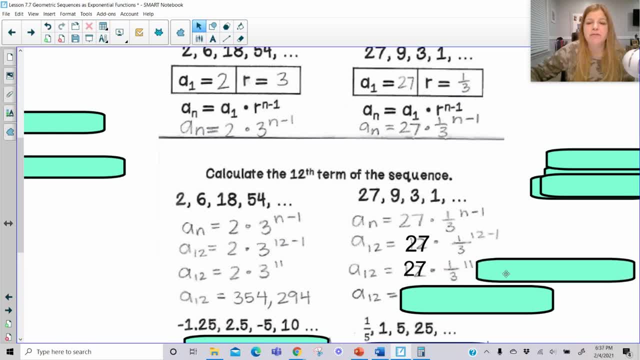 error here, So that's why I had to type over it. So this becomes 27 times one third to the 11th power. So now, if I take one third and I raise it to the 11th power, Now this is going to get a. 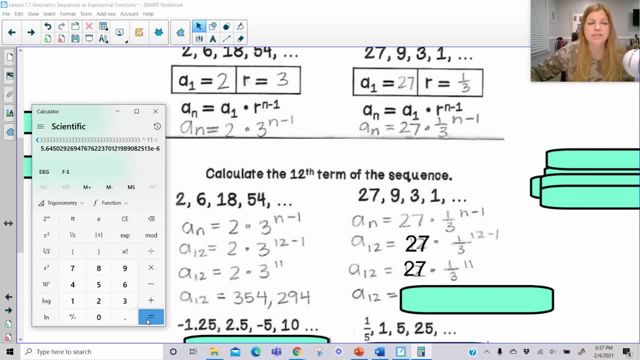 little messy because I am dealing with decimals. One third to the 11th power is really really small. You can even see in scientific notation: you have e to the negative six And then multiply it by 27. Again you get a really small number. Now, the way I kind of 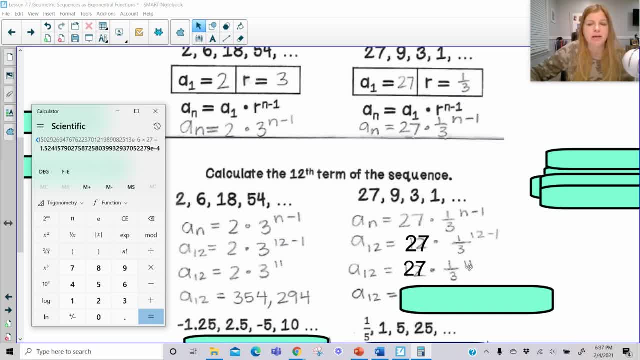 combated. this is, I figured well, 1 over 3 to the 11th. I'm sorry, one third to the 11th. Remember any fraction to an exponent? the numerator gets the exponent and the denominator gets the exponent. So what's 1 to the 11th power? 1.. What's 3 to the 11th power? Well, 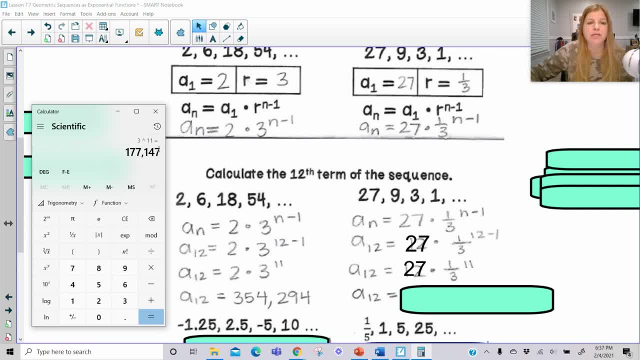 if I calculate that out, I get this number, And so this would be my denominator, 27 would be my numerator, And I'm just going to write it out like this: 27 over 177, 147.. Now this number, if I go to divide it by 27, is actually this value here? So I can simplify this. 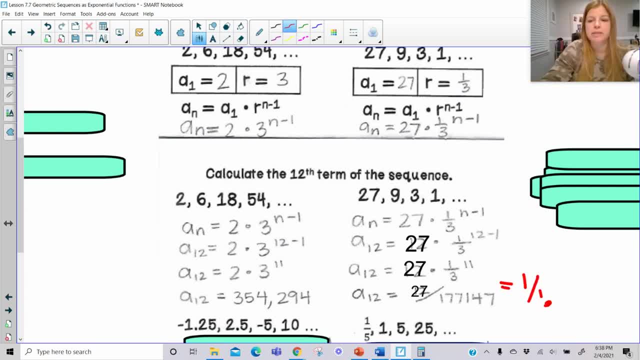 answer and it actually becomes 1 over 6561.. Okay, So what I did again is I changed one third to the 11th power, I made it 1 to the 11th over 3 to the 11th, and then multiplied it by 27.. And then 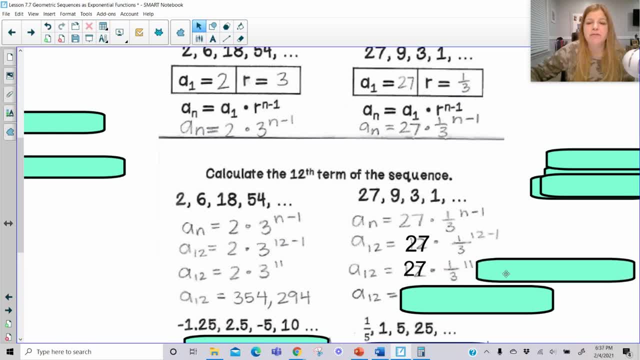 error here, So that's why I had to type over it. So this becomes 27 times one third to the 11th power. So now, if I take one third and I raise it to the 11th power, Now this is going to get a. 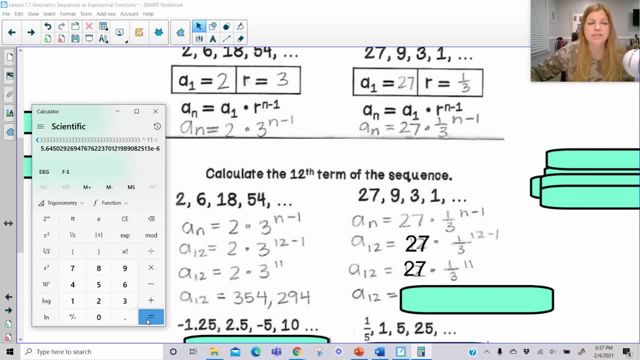 little messy because I am dealing with decimals. One third to the 11th power is really really small. You can even see in scientific notation: you have e to the negative six And then multiply it by 27. Again you get a really small number. Now, the way I kind of 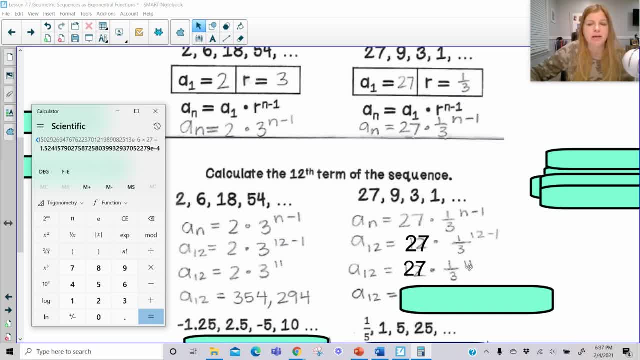 combated. this is, I figured well, 1 over 3 to the 11th. I'm sorry, one third to the 11th. Remember any fraction to an exponent? the numerator gets the exponent and the denominator gets the exponent. So what's 1 to the 11th power? 1.. What's 3 to the 11th power? Well, 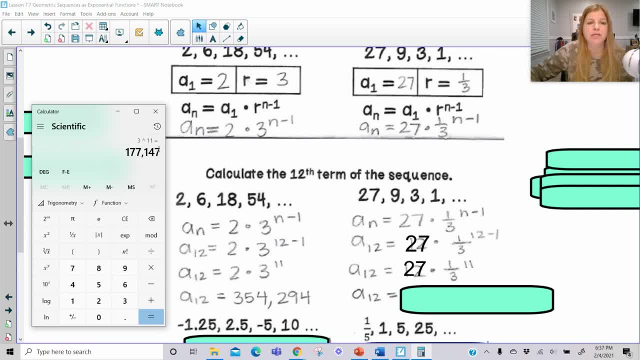 if I calculate that out, I get this number, And so this would be my denominator, 27 would be my numerator, And I'm just going to write it out like this: 27 over 177, 147.. Now this number, if I go to divide it by 27, is actually this value here? So I can simplify this. 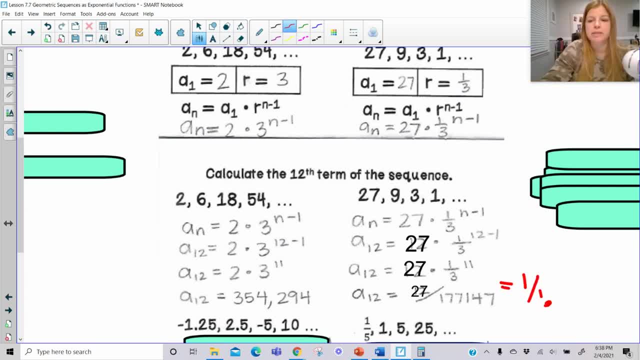 answer and it actually becomes 1 over 6561.. Okay, So what I did again is I changed one third to the 11th power, I made it 1 to the 11th over 3 to the 11th, and then multiplied it by 27.. And then 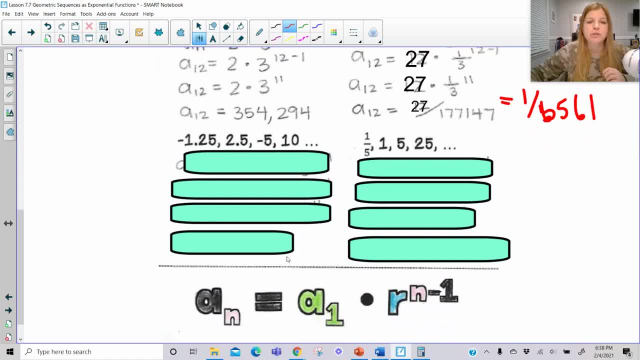 this actually does simplify out. Okay, Two last problems of this skill. So it's a sub n equals. you write the first term of the sequence times. what's my common ratio here? My common ratio is negative, 2 to the n minus 1 power. So then I want to calculate the 12th term. So a sub 12 is equal. 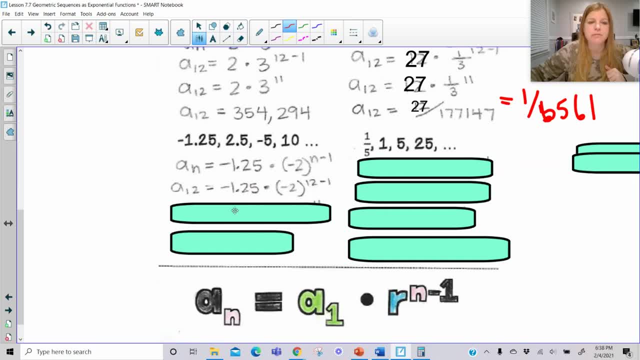 to negative 2 to the 12 minus 1 power. 12th term of the sequence is negative 1.25 times negative 2 to the 11th power, And again I'm going to guide you through. So we would do negative 2.. Now I'm 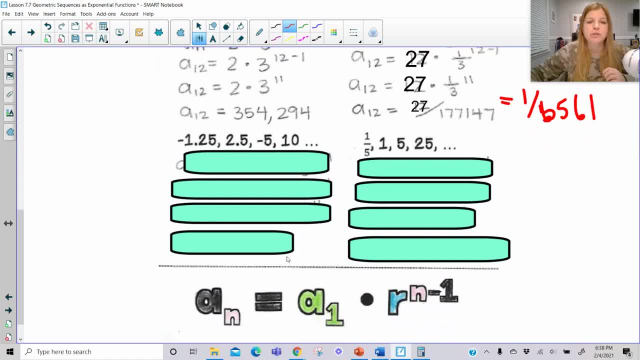 this actually does simplify out. Okay, Two last problems of this skill. So it's a sub n equals. you write the first term of the sequence times. what's my common ratio here? My common ratio is negative, 2 to the n minus 1 power. So then I want to calculate the 12th term. So a sub 12 is equal. 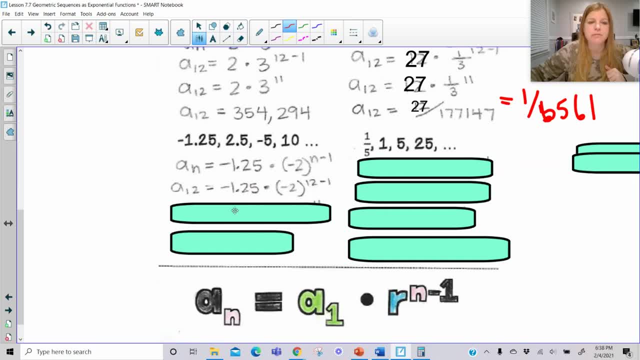 to negative 2 to the 12 minus 1 power. 12th term of the sequence is negative 1.25 times negative 2 to the 11th power, And again I'm going to guide you through. So we would do negative 2.. Now I'm 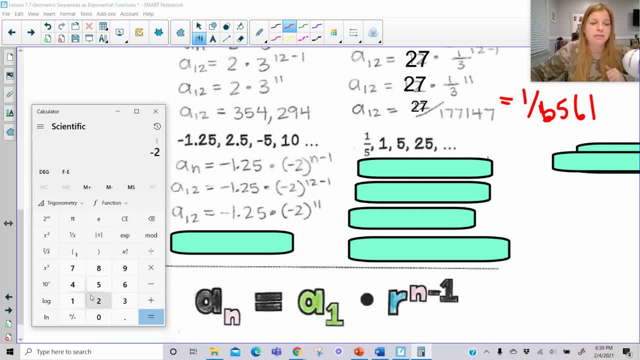 going to go ahead and put my negative 2 in parentheses. So negative 2 to the 11th power times, negative 1.25.. Okay, So I'm just going to show you that again in case you missed it. So you would do open. 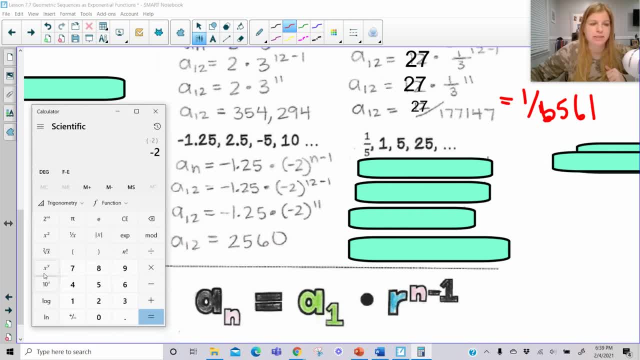 parentheses to make it negative. close parentheses X to the Y: 11, press enter times this negative: 1.25.. So you type in negative. I'm sorry you type in 1.25, make it negative, press enter. 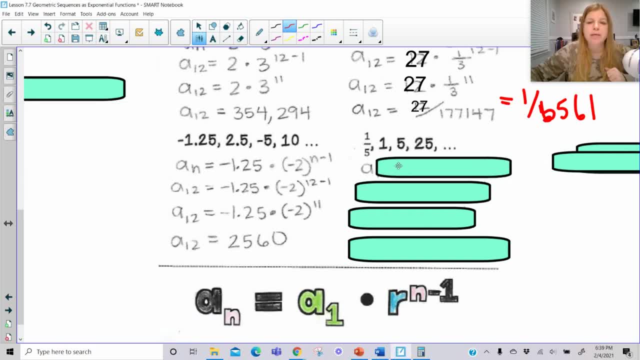 and that's our result. Last one, So this is going to be a sub n equals- it's the first term in the sequence- 1.5 times my common ratio. I see it's multiplying by 5 to the n minus 1. 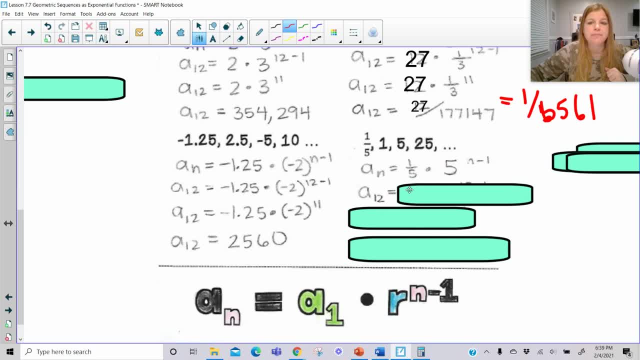 power. If I want to find the 12th term in the sequence, it's going to be 1.5 times 5 to the 12, minus 1 power. A sub 12 is equal to 1.5 times 5 to the 11th. So I would go here: 5 to the 11th. 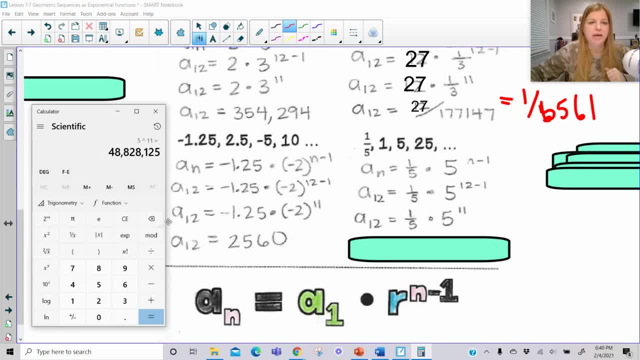 power And then times 1.5 actually just means the same as dividing by 5.. So you can type it in either way And I end up getting this pretty big number of 9,765,625.. I know there was a lot going on in. 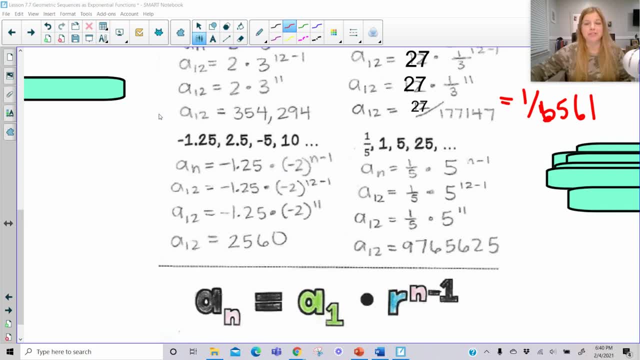 this video. I hope it was easy for you to follow along. Thank you so much for watching, Bye.